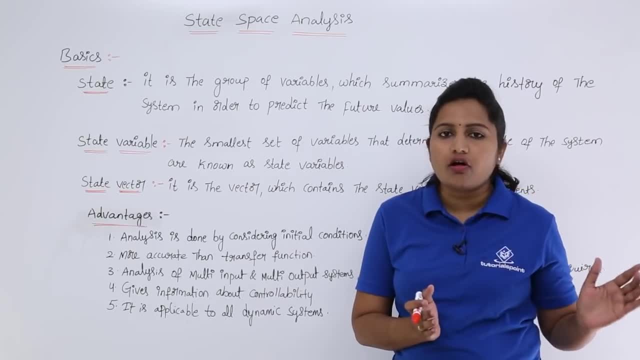 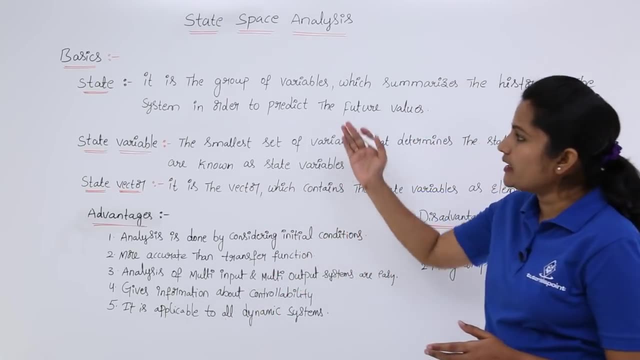 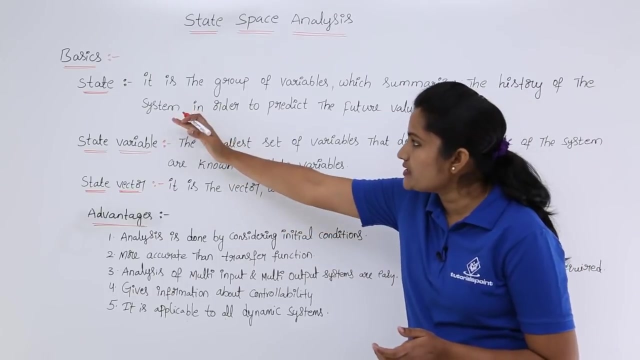 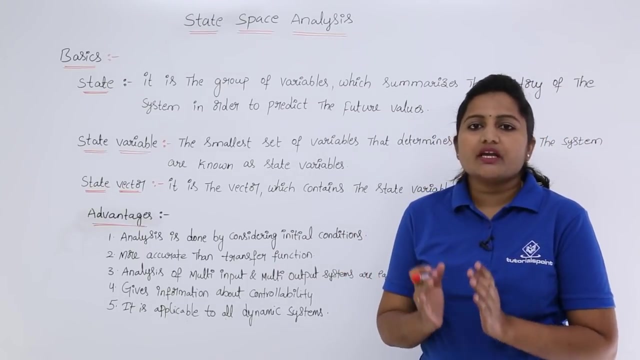 that is summation of all the history, all the previous values, which is supposed to predict the future value. So that is why, so we can say the state is nothing but group of variables which summarizes the history of the system in order to predict the future data. So here state is because of: 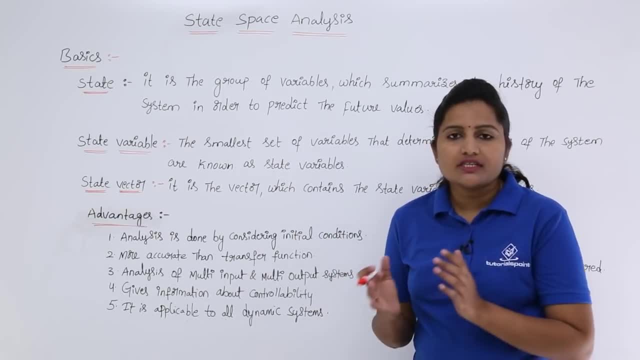 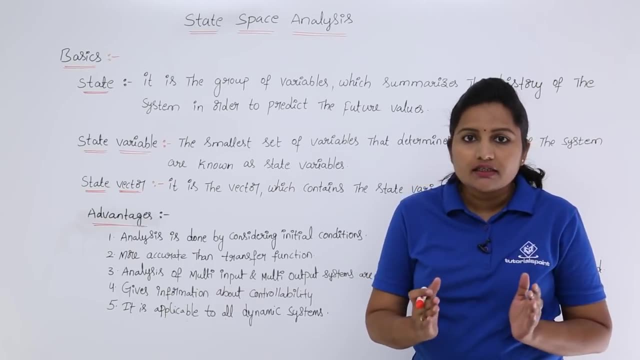 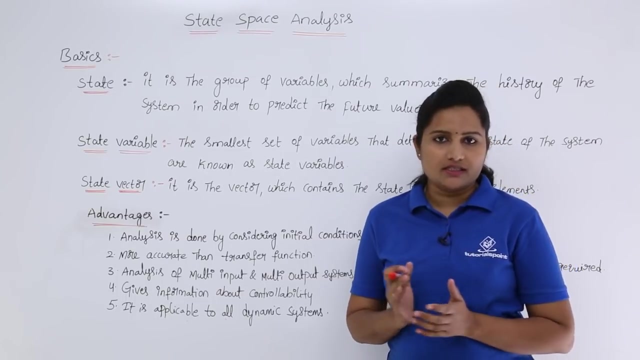 the history and used to predict the future. So this is nothing but state. Now we are in this state is because of our history and this state can predict our future value. So that is nothing but state of any system. For example, if you are having any dynamic system, 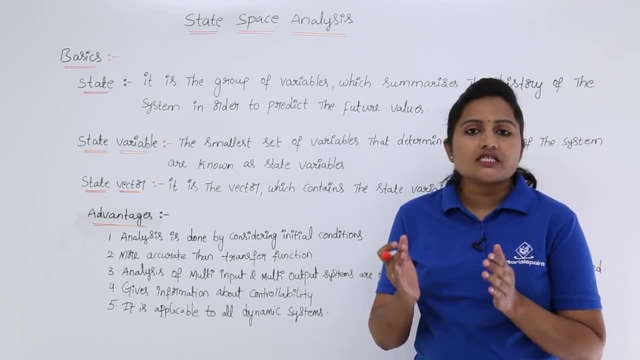 if you know the dynamic system, at t equal to t 0, that means at initial condition. if you know so that initial conditions came because of the history of that system And the system response at t equal to t 0, if you applied t greater than or equivalent to t 0 values. 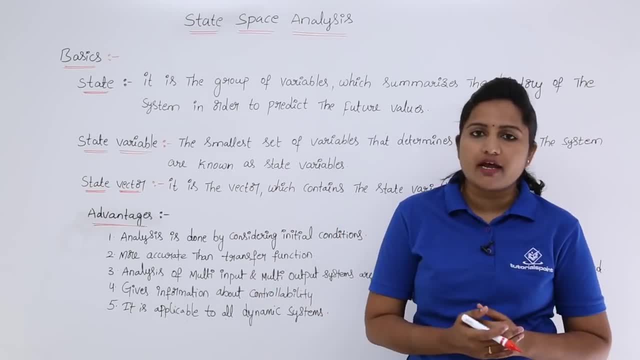 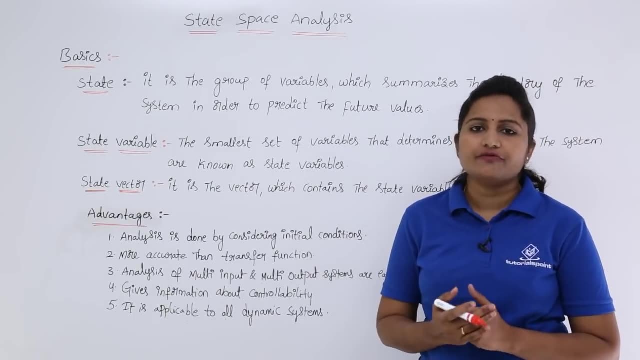 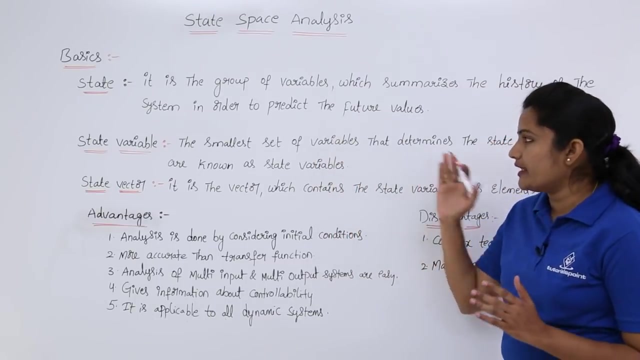 that by that value we can predict the future values of the system. So state is because of the history and used to predict the future value of the system. And coming to state variable, this is the smallest set of variables that determines the state of the system. So this is: 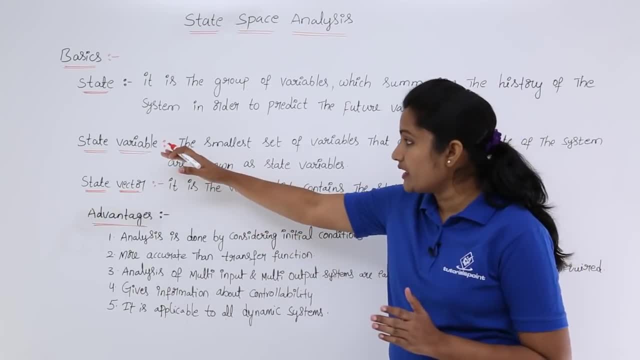 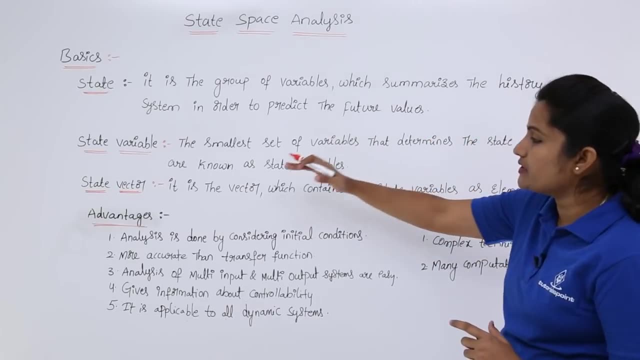 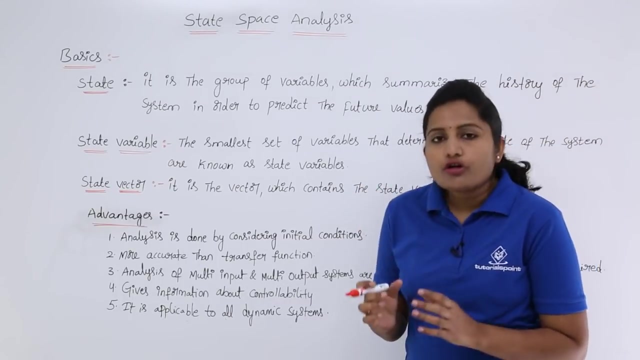 smallest set of state variables. we can say: state variable is nothing but the smallest set of variables. which variables? that variables determines the state of the system, or known as state variables. So, for example, if you want to determine a state of this system, if you want to 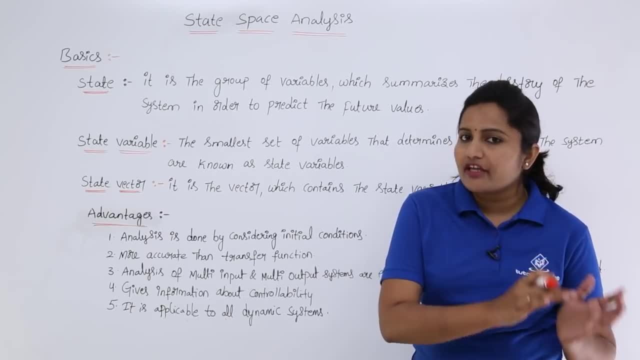 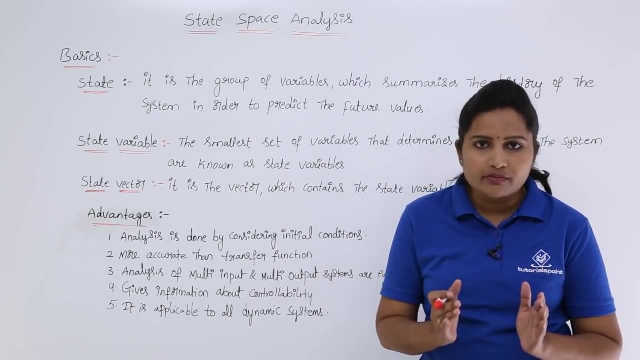 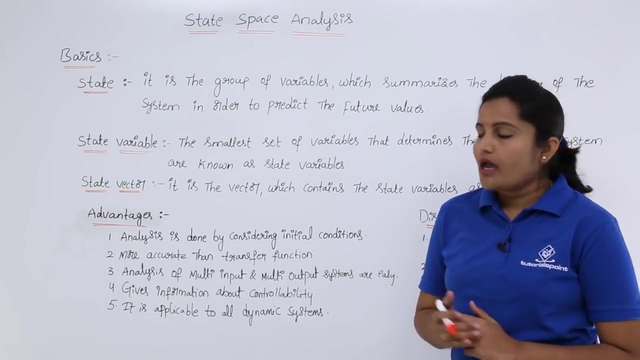 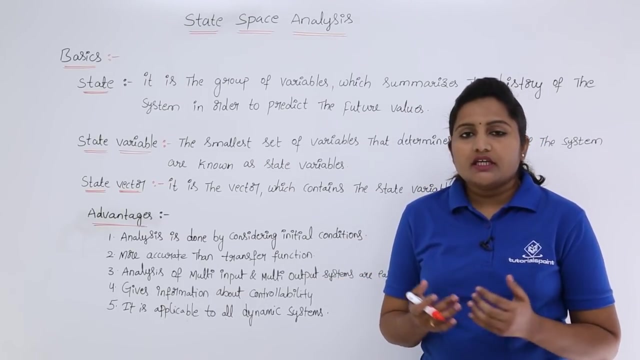 determine the state of the system. whatever the variables you require, that set is nothing but state variable. The smallest set of variables which used to determine the state of the system is nothing but state variable. And now here, for example, we can take in a capacitor, the 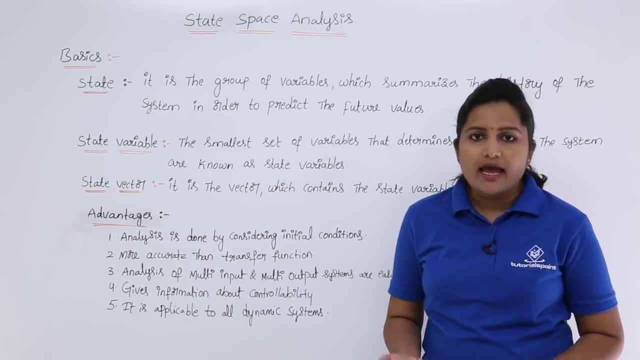 initial voltage of the capacitor we can take as state variable. Why? Because this came from history and that initial conditions or initial voltage of the capacitor, with that we can determine the state of the system. So like that voltage in the capacitor, initial voltage in the capacitor or initial current in the inductor we can take as an example. 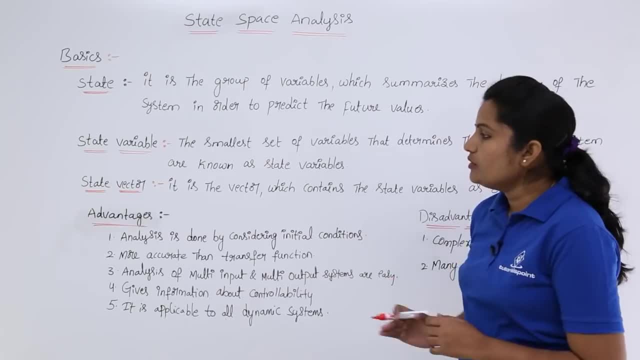 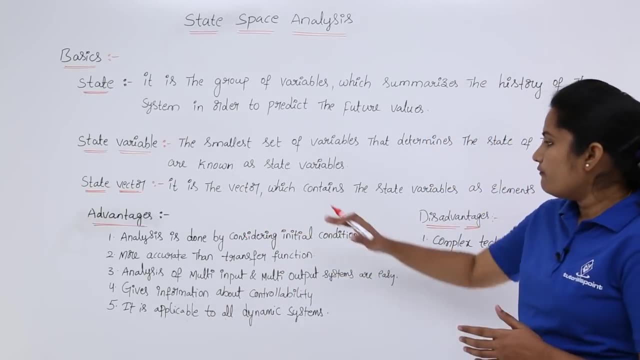 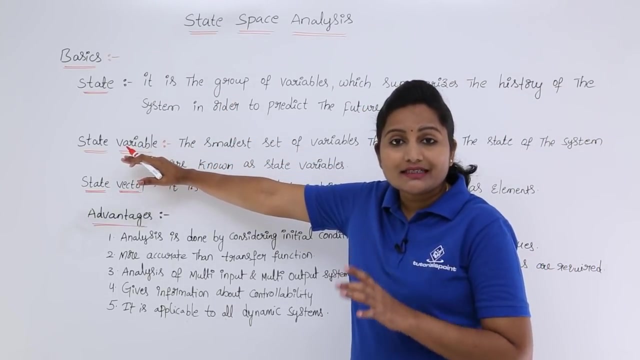 for state variable. And now we will get into state vector. What is meant by a state vector? It is the vector which contains the state variables as elements. So here state variable is nothing but the set of variables which determines state. Here state vector is nothing, but it is the vector. 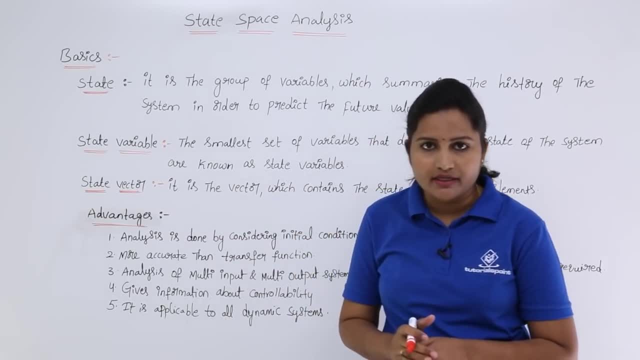 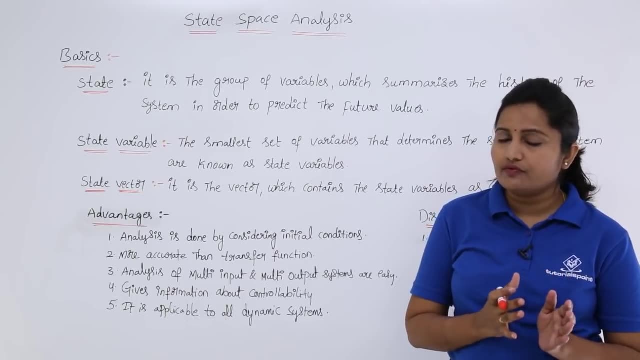 which contains state variables as its elements. If a vector contains state variables as elements, then it is a state vector. So this is the state vector, So this is the state vector. Then we can say that is a state vector. For example, if you take in capacitor, the initial. 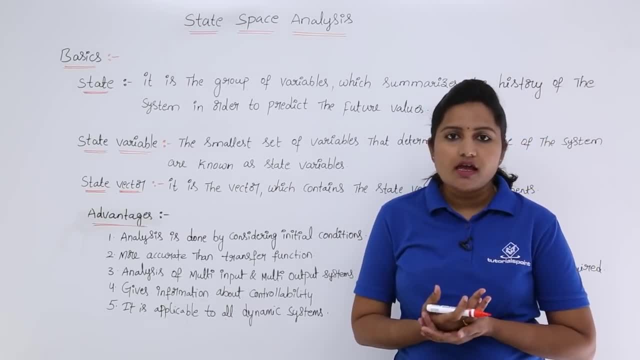 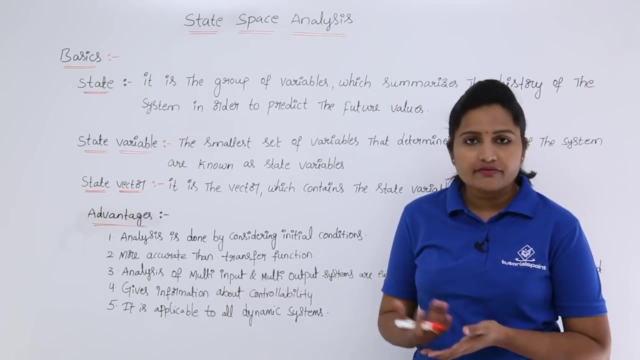 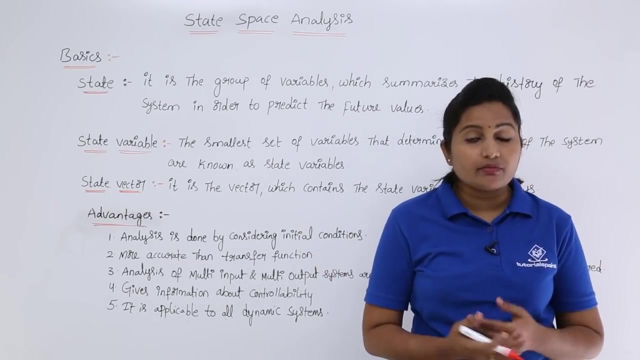 voltage of the capacitor can be treated as a state variable and the current initial current in a inductor can be taken into an example for state variable. If you are having those two variables in a vector, you can say that is a state vector, because the vector 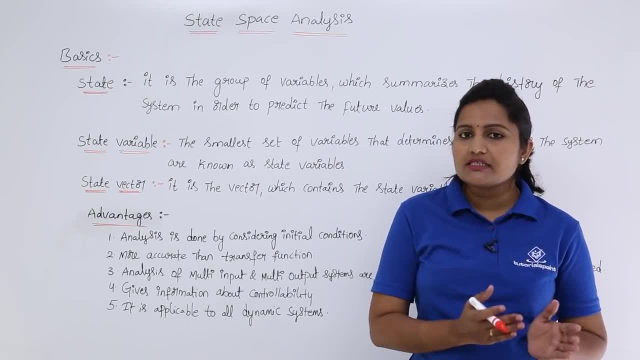 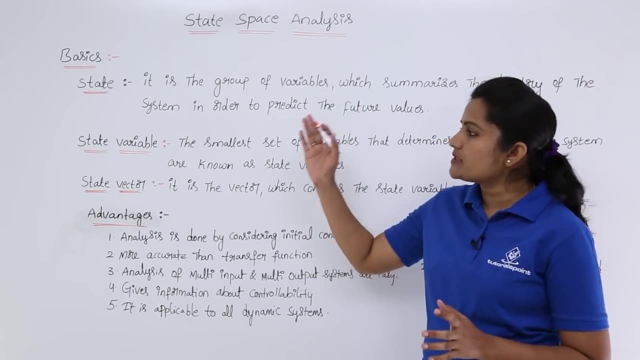 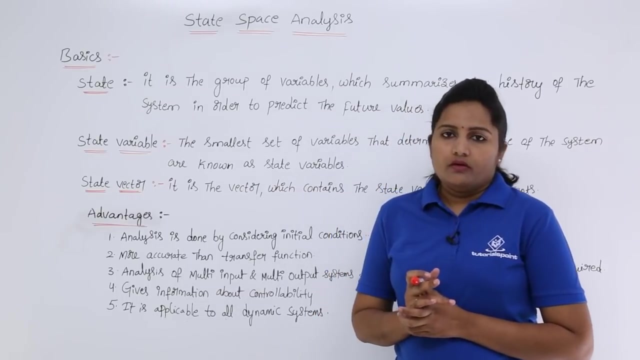 contains elements or state variables. So that is why we can say that vector as a state vector. We got an idea, simple idea, about what is meant by state and what is meant by state variable and what is meant by state vector. Now we will see advantages and disadvantages. 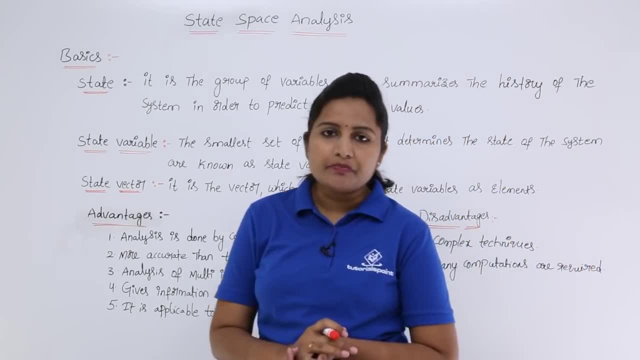 of state space analysis, As we are having transfer function techniques and before in control system. 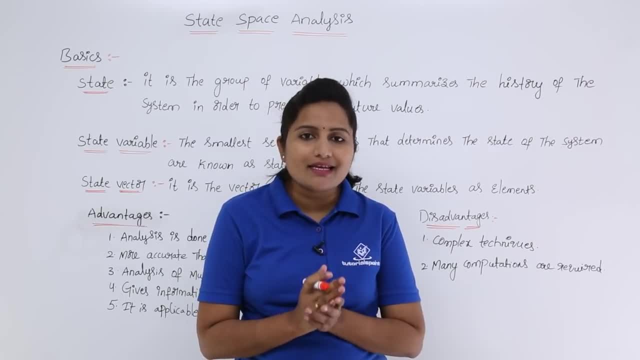 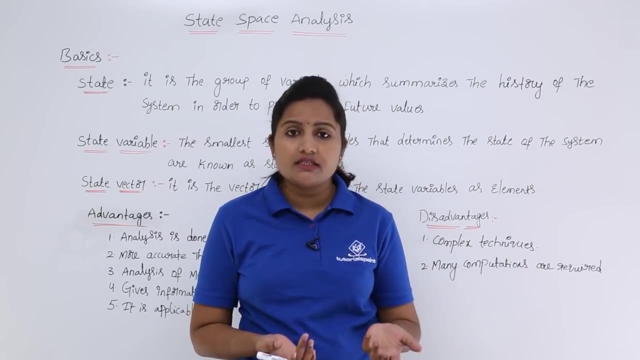 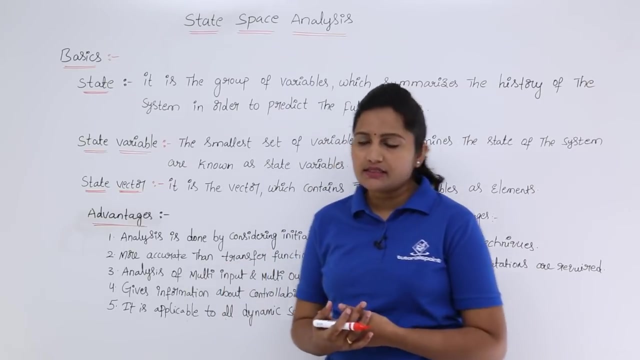 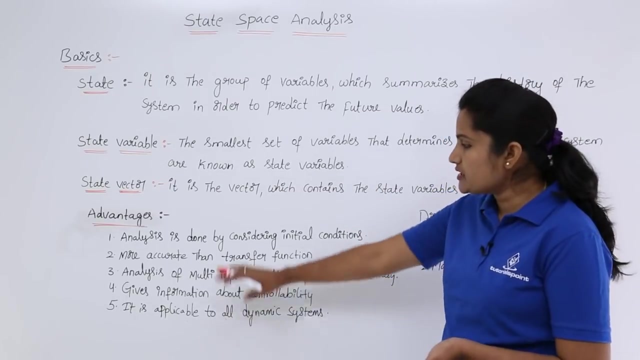 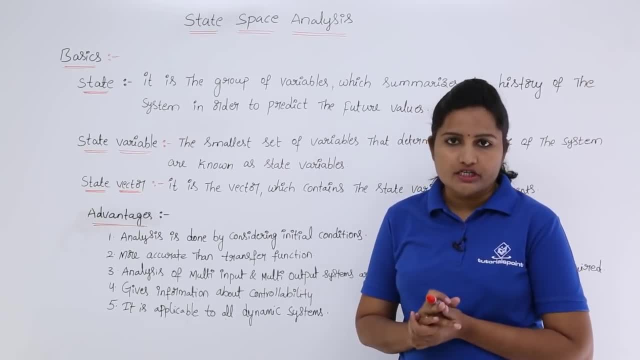 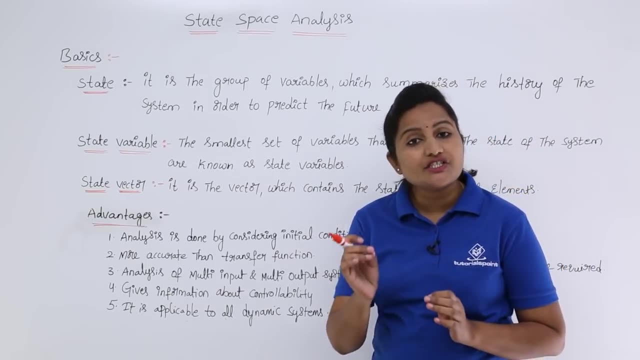 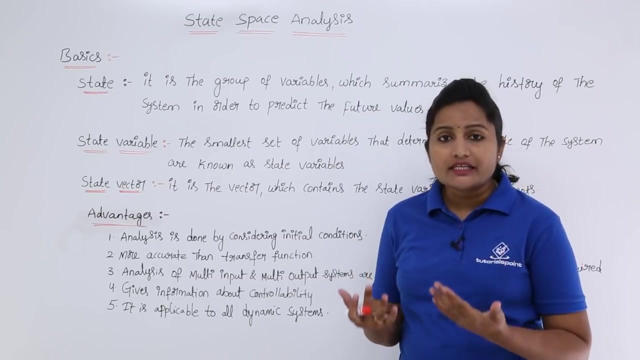 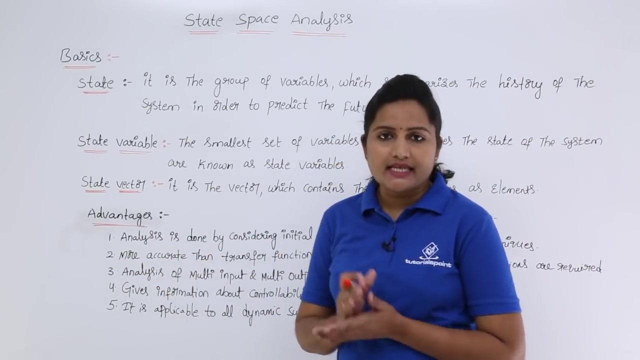 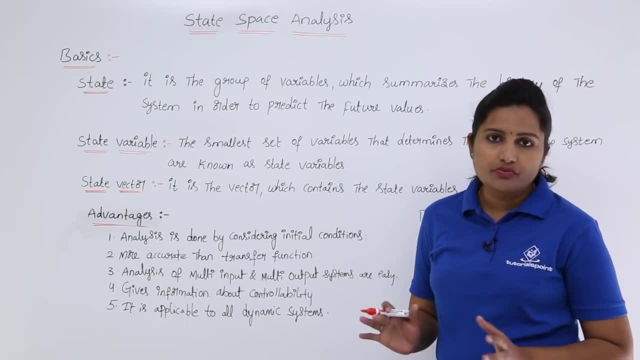 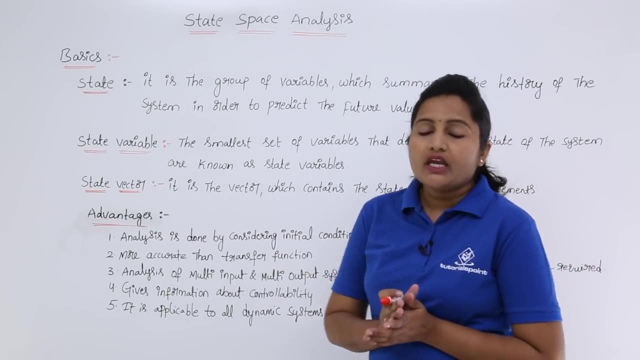 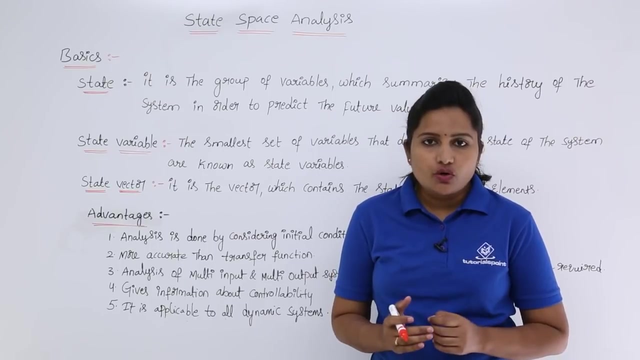 based on initial conditions. So this is one of the advantage we can take and more accurate than transfer function techniques. Up to now, in so many techniques to analyze the system, we have considered the transfer function forms. So whatever the results, there you are getting. 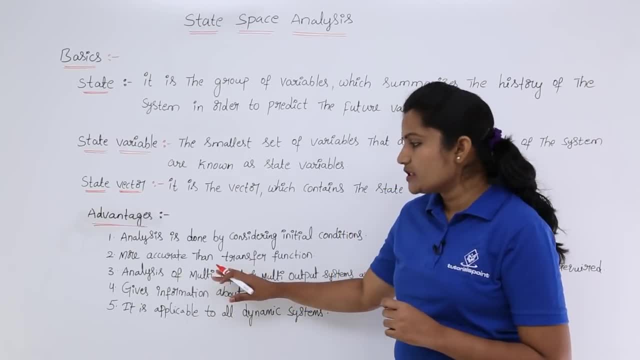 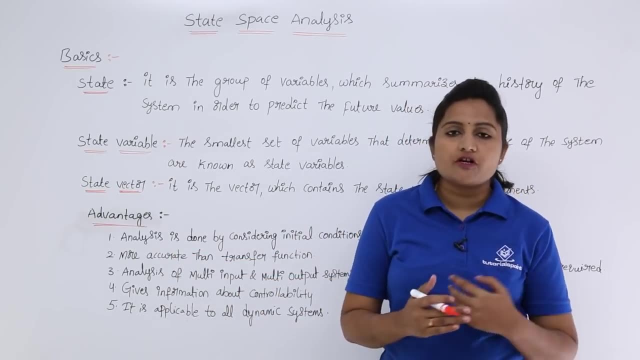 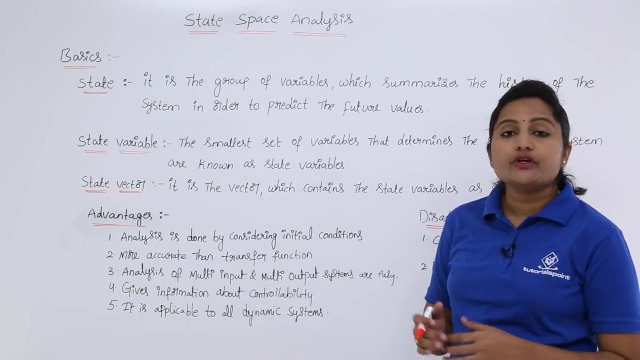 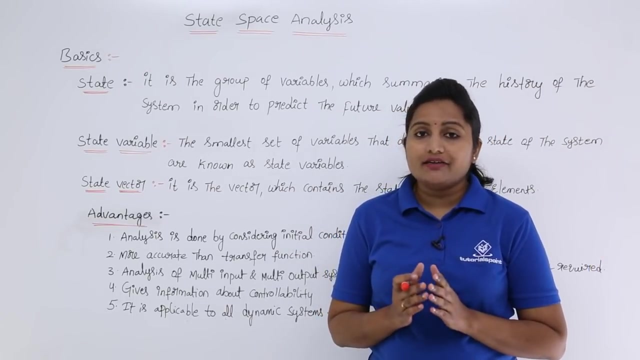 for analyzation of system. compared to this, this one is more accurate. This will provide more accurate analysis compared to transfer function related techniques. So now coming to third advantage: analysis of multi input and multi output system will be made easy by this technique If you are taking transfer function, if you are having single input and single output. 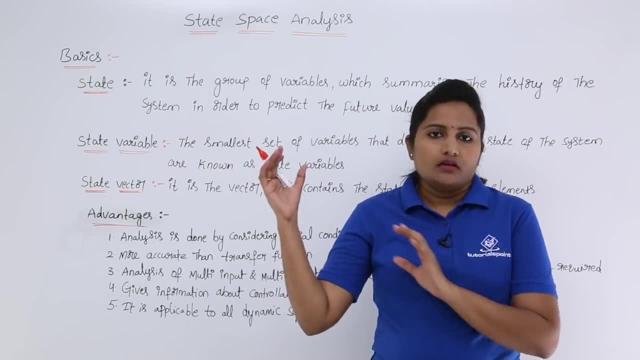 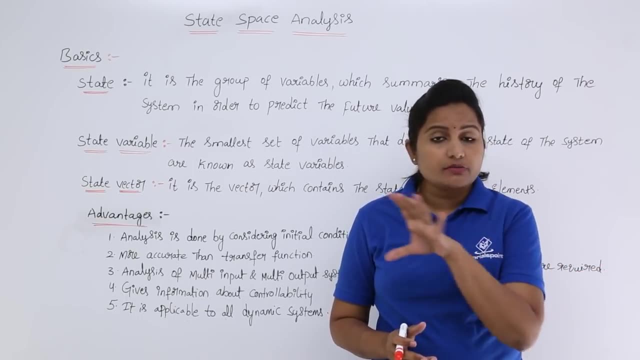 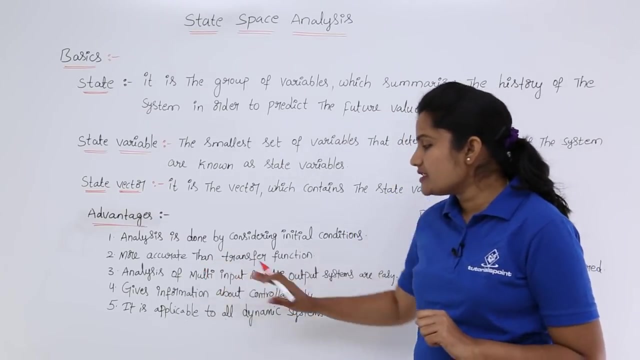 transfer function is nothing but Laplace transform of output by Laplace transform of input If you are taking single input and single output. transfer function is nothing but Laplace transform of input If you are having multiple inputs and multiple outputs. this transfer function techniques may not be easy, but here analysis of multi input and multi output systems are. 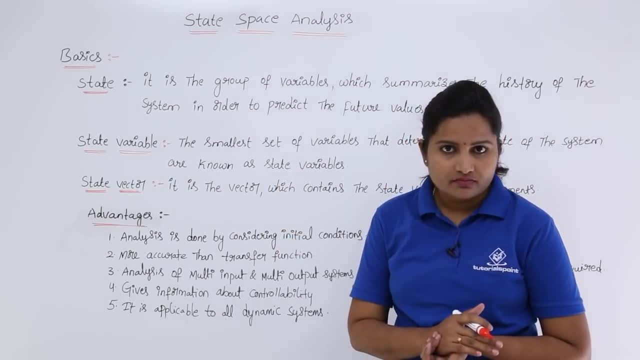 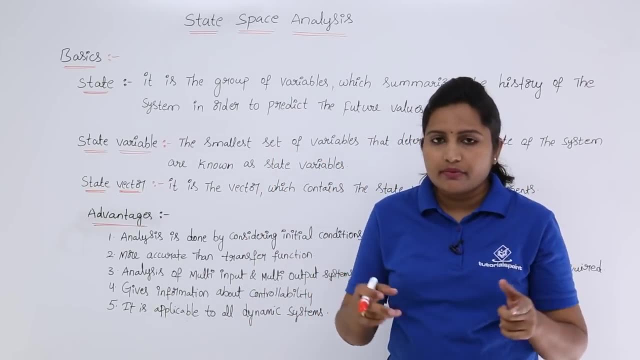 very easy as we are having state vector, So we can take all inputs as vector and we can take all outputs as vector. So that means so we can take like a matrix. So that will get into the analysis when we get into the analysis. 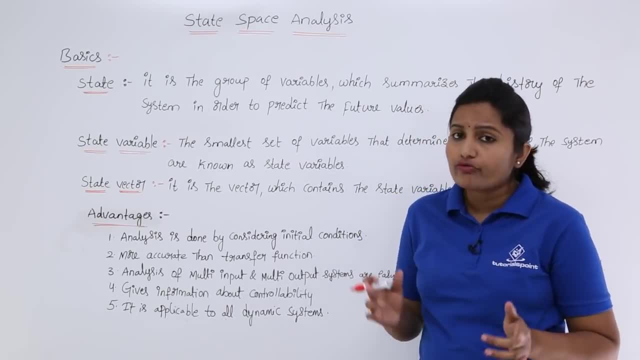 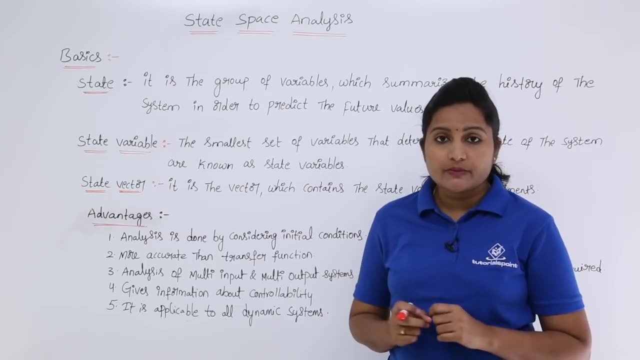 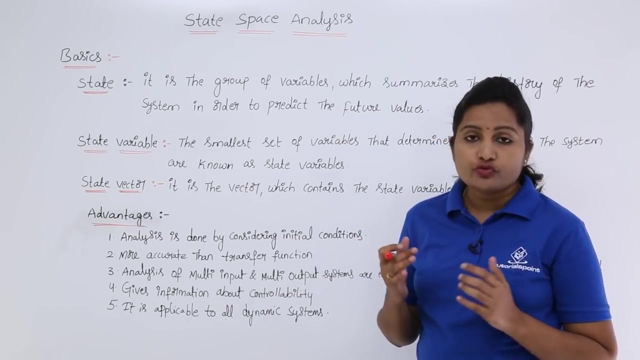 Then you use it to get the data how we are dealing with multi input, multi output systems. this is very, very important. By this state space analysis, we are making easy of analysis of multi input and multi output systems. So which is having two are more inputs and two. 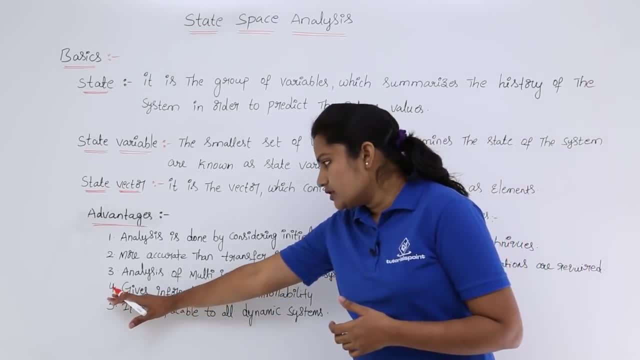 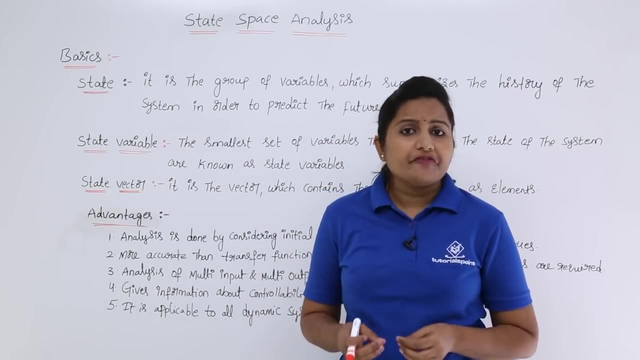 are more outputs. And here, coming to another advantage, gives information about controllability. This is very important for your control system, control system. By this analysis we can say how how much extent a system is controllable, how much extent it can control it functionality. 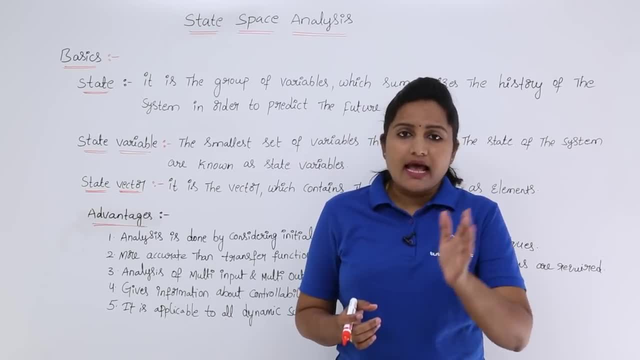 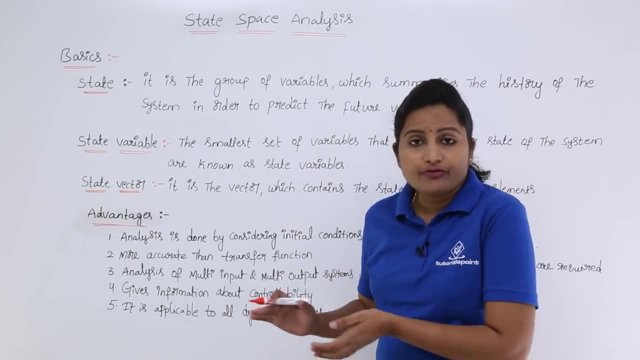 or how much extent this having observability. So all these will come with this state space analysis. it will gives you an information about the system, that how much it can therefore control its concerns. So this is theопрос, this is your injury or death information. I. 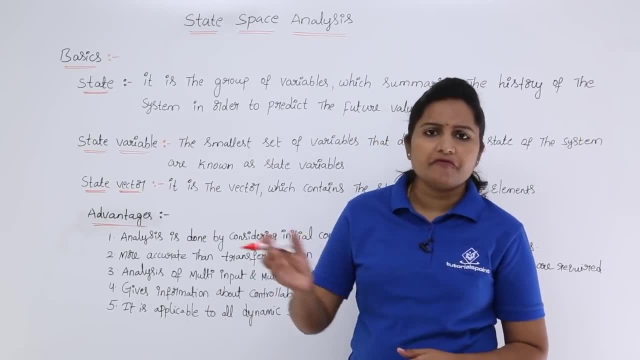 thus didnot know these word control information that hopefully it is根prest quais to know. Now let us see what the threshold of a watcher style. So if a try CASP match conditions in CSS extent, that is controllable how it can perform. So this is one more advantage by state space. 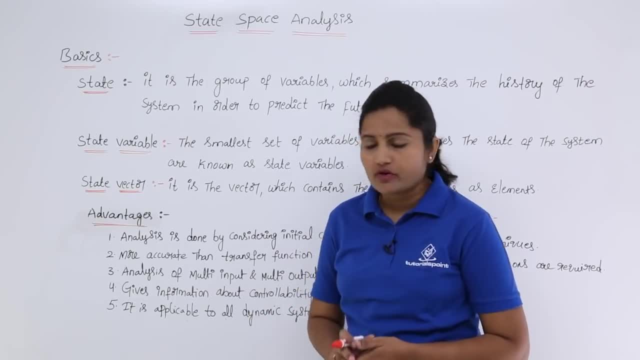 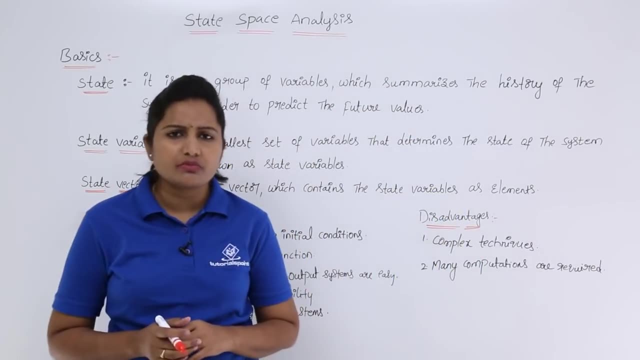 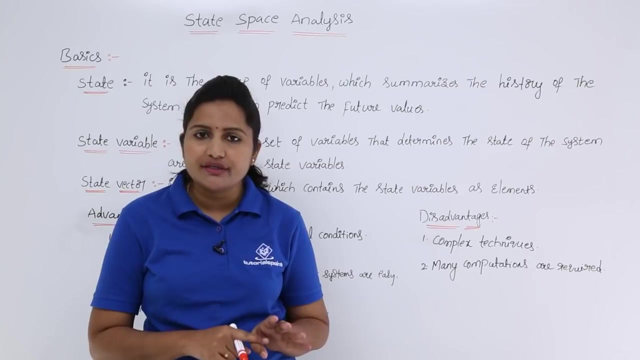 analysis. And coming to another important advantage, it is applicable to all dynamic systems. It is applicable to all dynamic systems means: if you know this analysis, you can analyze all dynamic systems. Dynamic systems means linear system, non-linear system, time variant system, time invariant system. all these are dynamic systems. So if you know state. 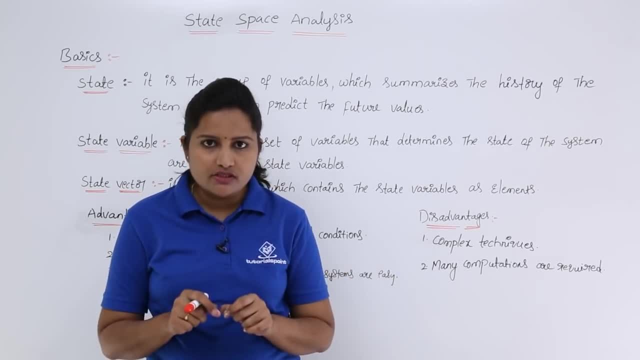 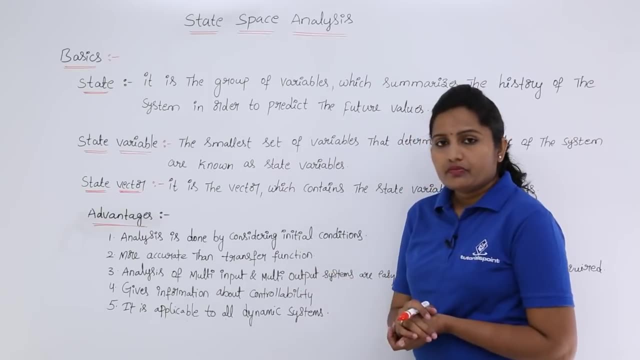 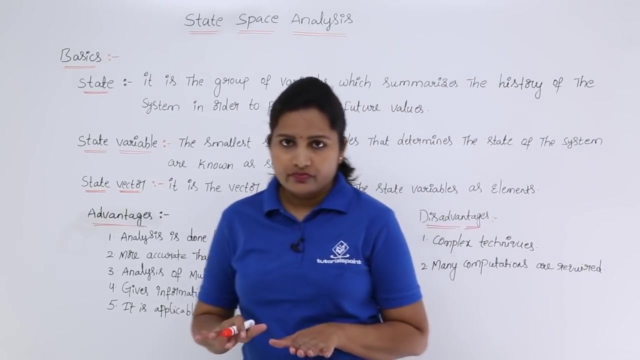 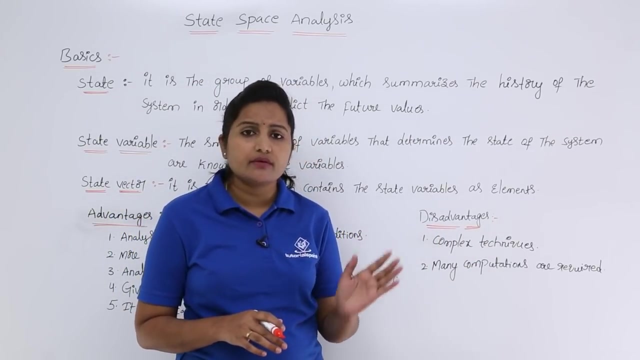 space analysis. any of these systems, any of these four dynamic systems, you can analyze. So now, here, as you are having so many advantages like that, you are having disadvantages too. So these two are the disadvantages: complex techniques. But here, as we are dealing with multi input, multi output, or we are using some vectors and matrices,